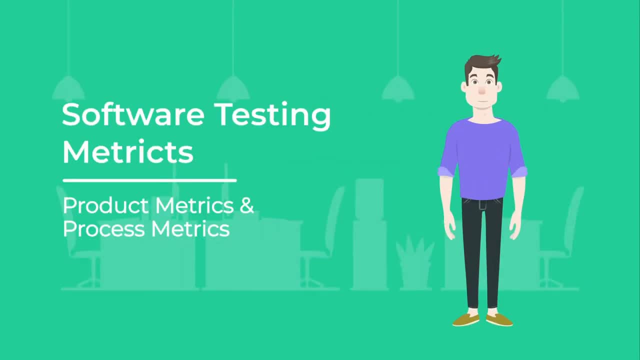 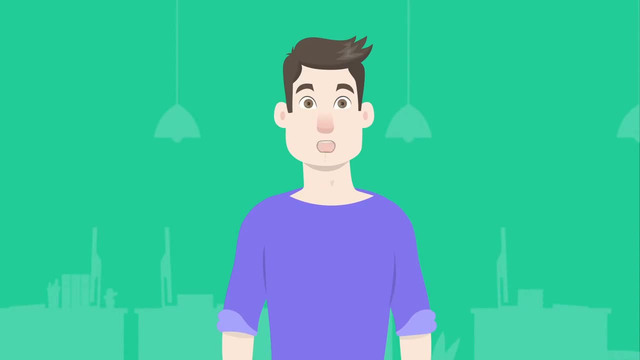 QA Metrics- Software Testing Metrics. QA metrics are used to estimate the progress and effectiveness of testing activities so a team can plan their working processes efficiently. In this video, I will tell you about the different types of metrics and how to use them. There are base metrics: 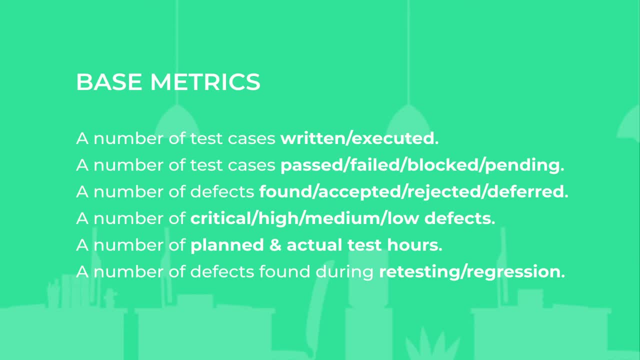 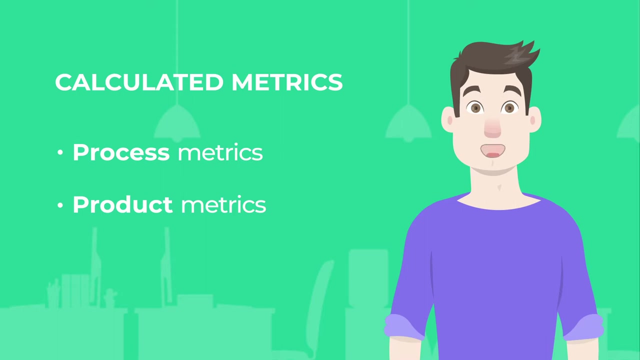 also known as absolute. They encompass various measurements gathered during test case development and execution. On the screen, you can see a list of QA base metrics for tracking your project. The other group is known as calculated metrics or derivative metrics. This data allows you to estimate the effectiveness of the testing process and the quality of the. 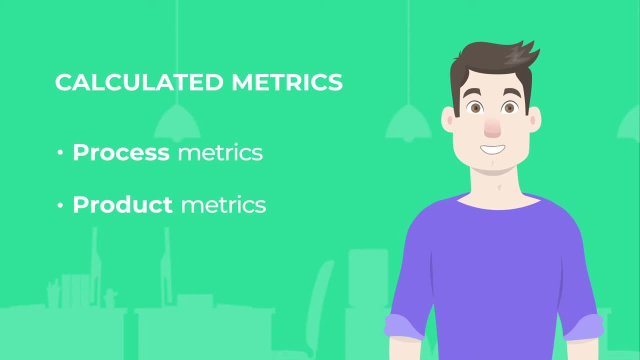 product under test To get calculated metrics. QA leads and team managers apply specific formulas to previously collected base metrics. There are two types of calculated metrics: process and product ones. Let's take a closer look at each of them. QA Metrics- Process metrics- are used during test preparation and test execution. 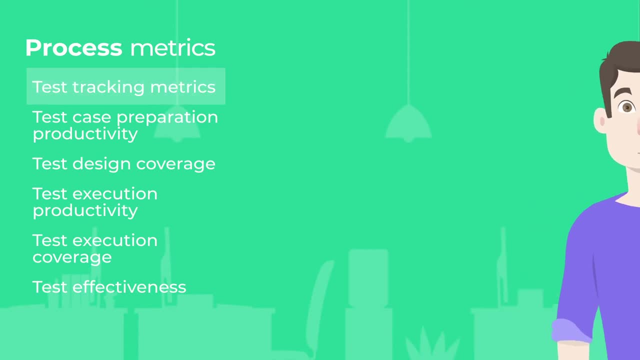 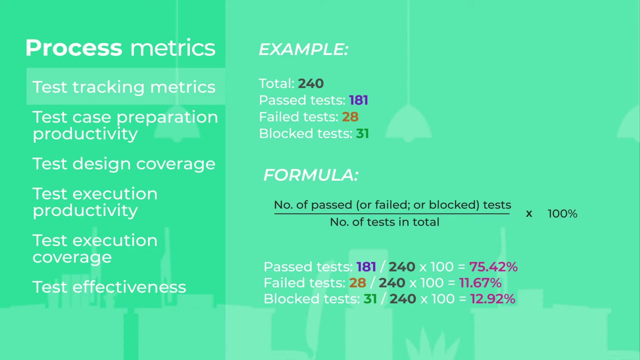 Here is a list of metrics that belong to this category: QA Metrics, Test tracking metrics show the percentage of passed, failed, blocked tests, etc. Let's take a closer look at it. For example, we have 240 test cases in total, 181 of them passed, 28 failed. 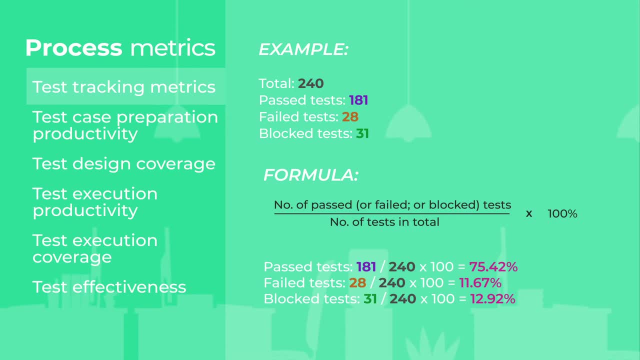 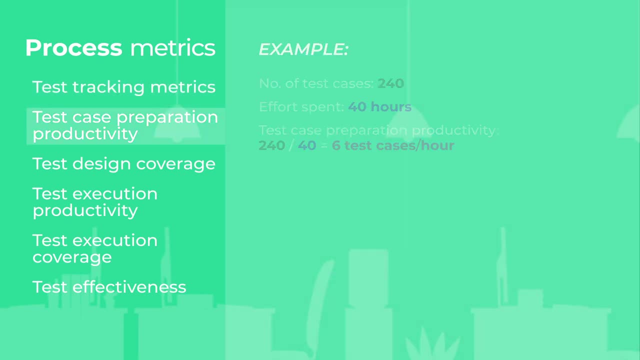 and 31 were blocked. To calculate the percentage of passed tests, you have to divide their quantity by the total number of executed tests: Test Case Preparation Productivity. Then goes test case preparation productivity. It is a way to estimate the timing of test case. 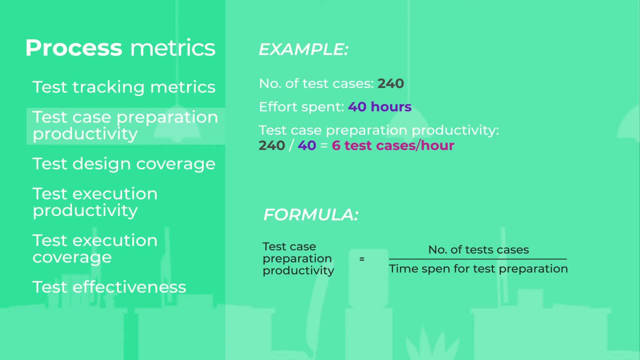 preparation. In other words, you will get test cases per hour ratio, just like the one on your screen. Test Design Coverage: Test design coverage is used to measure the percentage of requirements covered by test cases. Here's an example: Test Execution Productivity. 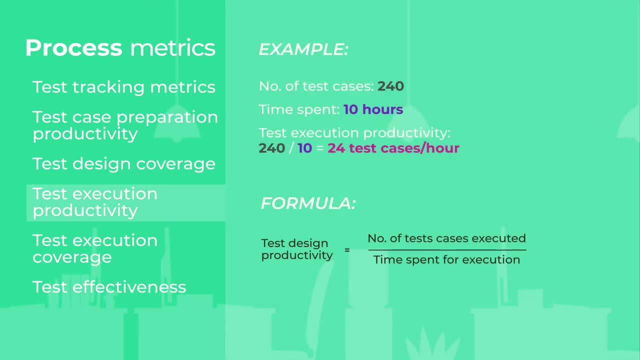 Test execution productivity shows how many test cases that can be executed per hour. Test execution coverage helps to track the progress of testing activities by comparing a number of already executed and planned tests. Here is a formula you can use. Finally, test effectiveness allows you to estimate the value of a test set.